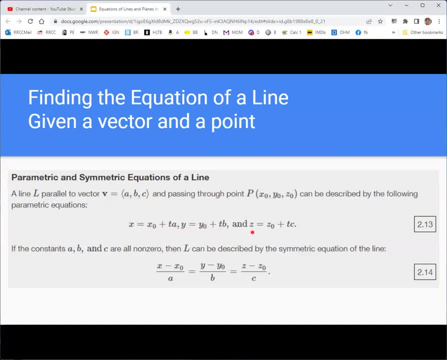 over 10.. 10. 10. you have an x equation, a y equation and a z equation, And each one of these equations is a linear equation for the variable t, which is the parameter, And the way I like to think about these, or remember them, is to think of a linear equation of two variables. 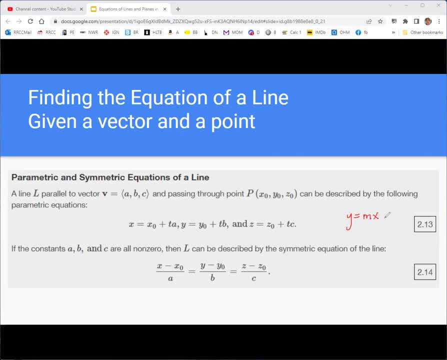 Everybody probably remembers the slope-intercept formula. y equals mx plus b, So x. your independent variable is being replaced by the parameter t in each one of these And the slope number m is different for each of the directions. So it's a, b and c and these are the components of the vector. 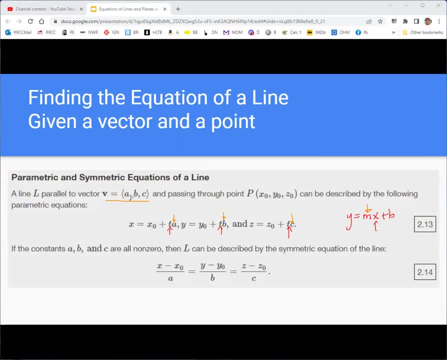 And the vector tells you which direction and sort of the tilt of the line. So it makes sense that the components of the vector are like the slope numbers in these equations And the last part, the y-intercept, the constant that's added on there. 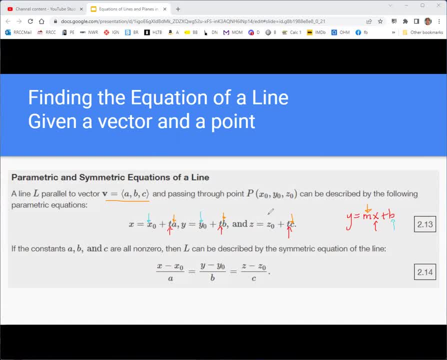 those are the coordinates of the point that you're using. So here they're x-naught, y-naught and z-naught, And those are the three coordinates of the point, which is sort of your starting point for when the independent variable is zero, right. 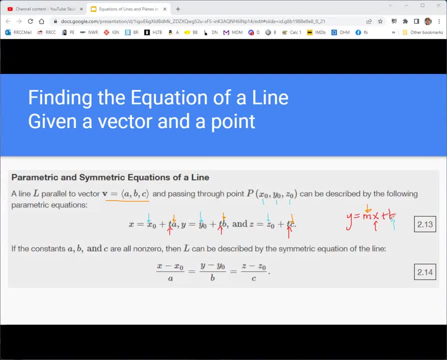 So when t is zero, you're at that point, p in the y equals mx plus b equation. when x is zero, you're at y equals b. So I think of that format and hopefully understand those three equations. Now the same line can be represented as one three-part equation. 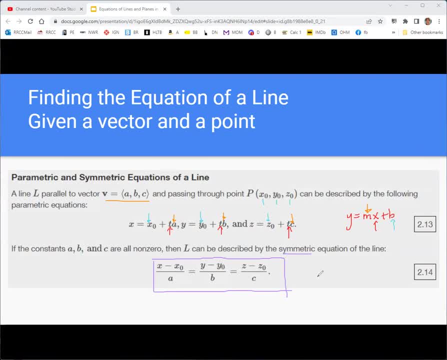 And this is known as a symmetric version. So you have your parametric version and your symmetric version, And you'll notice that t is not here. In fact, that's how you get from one equation to the other. is you take any? 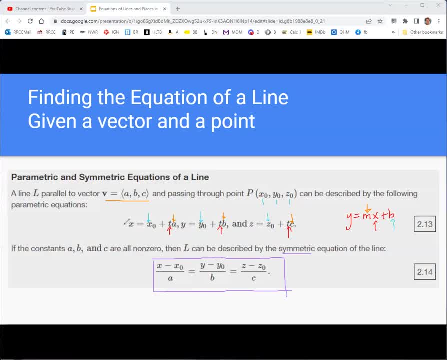 or you take all three of the parametric equations and solve for t. So we can do that with one of them. If I just solve this for t, I would subtract the x-naught and then I would divide by a, And you can do the same thing for the others. 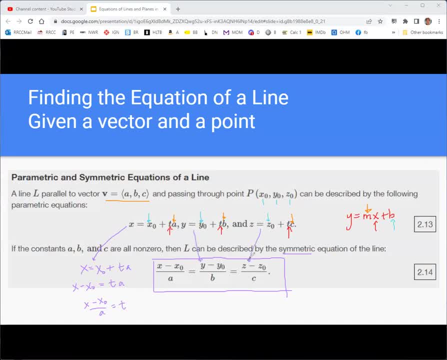 and you'll get a similar equation. And all those equations are equal to t. they're all equal to each other, And so you've eliminated the parameter to get just an equation with x, y and z. So a, b, c, x-naught, y-naught and z-naught are the same in both sets of equations. 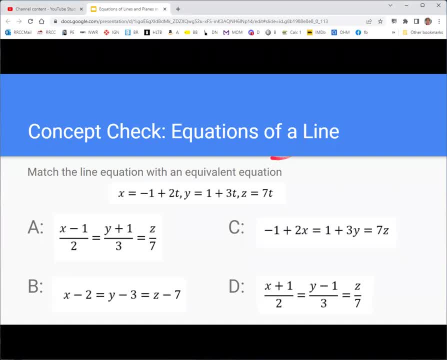 A quick concept check here to go from the parametric equations shown here at the top to the equivalent symmetric equations a, b, c or d. Take a minute to pause the video if you need some time, And I believe the correct answer is answer choice d. 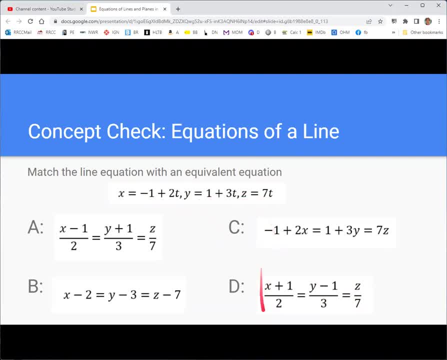 where you would just solve each of these equations for t and you should get the fractions shown in answer choice d, And they're all equal to t. so they're all equal to each other. So the correct answer is d. Now this is the same symmetric equation of a line. 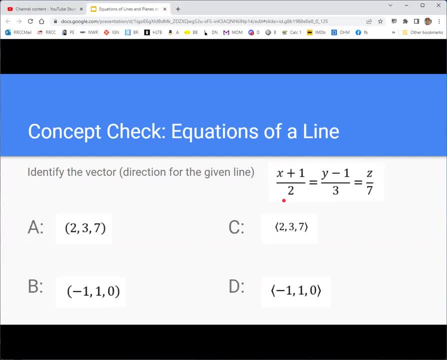 Let's see if you can identify from the choices here the vector that determines the direction for that line. And you should have found that answer. choice c is the correct answer. So remember, in this metric form of the equation of a line, it's those denominators that are the components of the vector a, b, c. 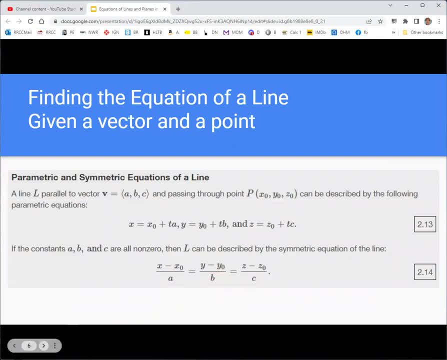 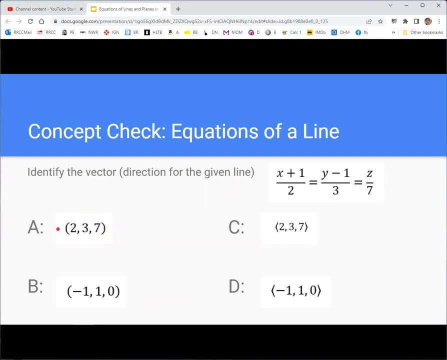 And you see that here in this definition. So 2,, 3, 7.. Now, a could be correct if you use parentheses. We're trying to avoid using parentheses for vectors because it's confusing, because that's the notation for a point. 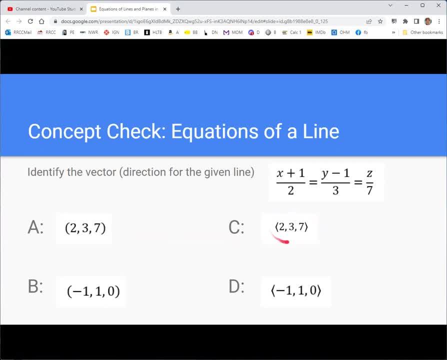 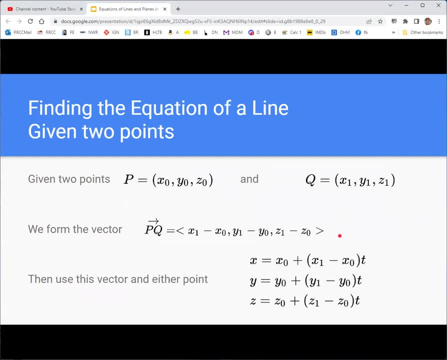 So I would prefer you use the bracketed notation for vectors when describing vectors. So if you were given two points instead of given a vector and a point and you wanted to get the equation, you would simply take the two points and form a vector. 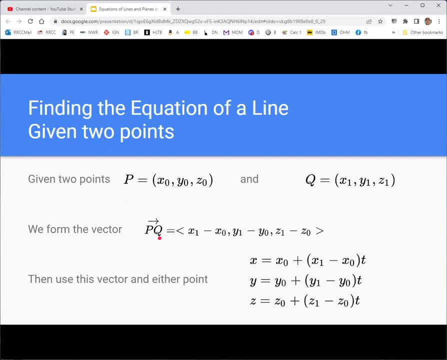 The vector from initial point p to terminal point q is just going to be the difference between the coordinates, And you do a terminal point minus initial point for each coordinate And I'll get you three coordinates, So that becomes your a, b, c, your components of your vector. 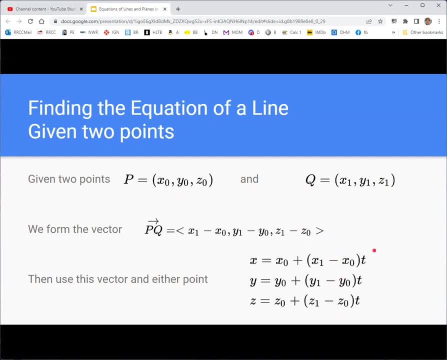 And that would just go in the parametric equations in front of t, And then you could use point p for your point, or q, either one. Here we're using point p, And since you can use either point, the parametric equations aren't unique. 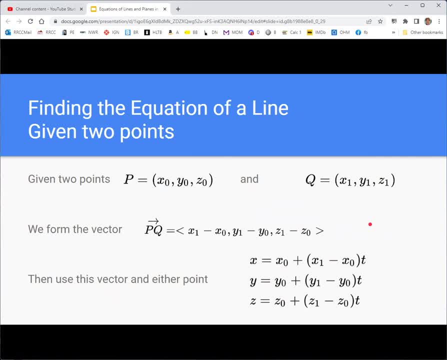 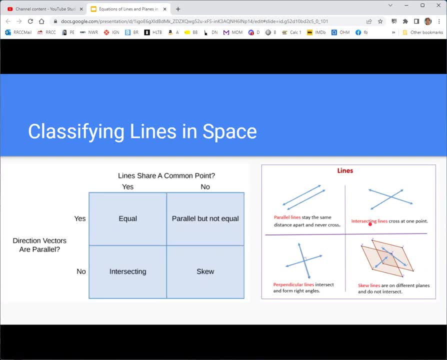 They can look different depending on which point you use, but should be equivalent. Now, if we have multiple lines, we might want to know their relationship with each other, And we can have the lines either be parallel, in which they don't cross and they have some set distance. they are apart. 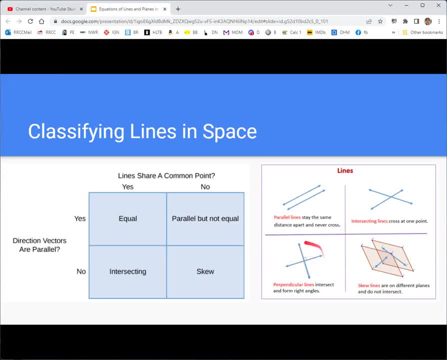 or intersecting, where they cross at a single point. Perpendicular lines intersect and form right angles. That's a specific case of intersecting lines, But in three dimensions. there's another case That's not parallel or intersecting and that's skew. 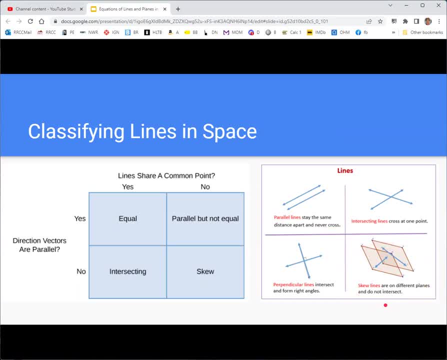 And you can't have this in two dimensions. In two dimensions, lines are either parallel or they cross. But here, if the lines are on parallel planes, the lines aren't necessarily parallel, but they won't actually intersect, because the planes don't intersect. 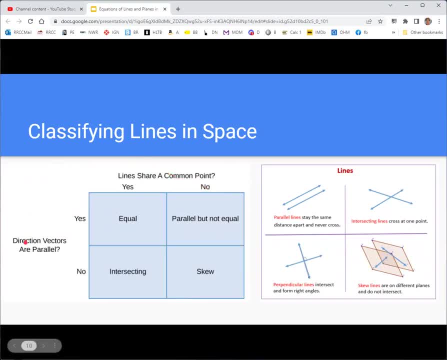 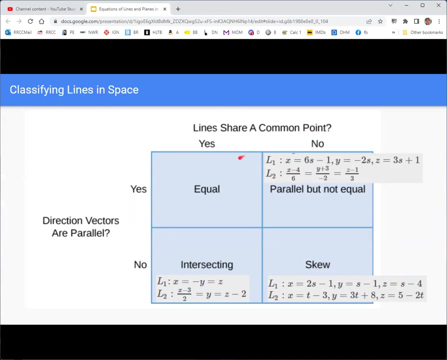 This table here summarizes the connection between the vector and point and whether they're parallel intersecting skew, Or again you could have them be the exact same line. So if the two lines are equal, then the equations should be equivalent. Maybe one is multiplied by a constant in all the parts. 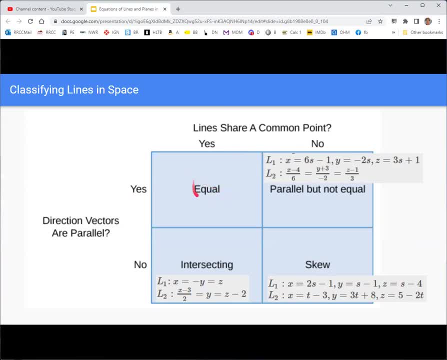 and that would still be equivalent. But it should be pretty obvious that they're equivalent If they're not. parallel would be the next easiest thing to spot. And what you're looking for there is that they have the same vector, So the direction vectors would be the same. 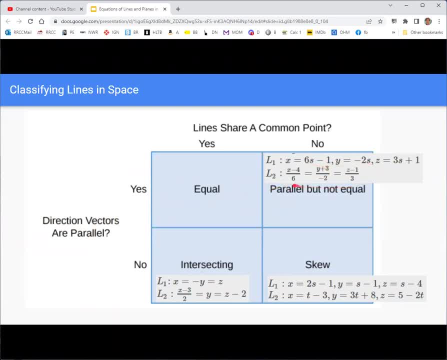 And so the numbers for A, B and C would be the same in both lines. And you see here this L1 line has the parametric equations using S as the parameter, So it's not always T, You can use a different letter. 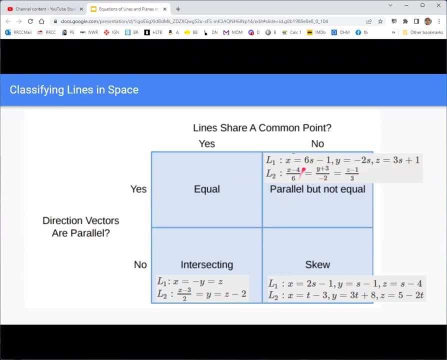 And then the symmetric equations for the second line, L2,. but you can still tell that A is 6,, B is negative, 2, and C is 3.. And then, if you look closer, you'll notice that the other numbers are different. 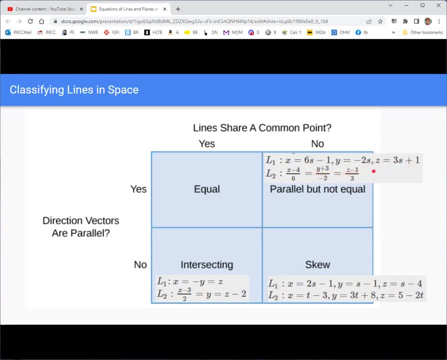 The numbers for X0,, Y0, and Z0. And therefore the lines are not equal right Because they don't have that same point. So there would be a case of parallel lines And when you look at the intersecting and skew cases, 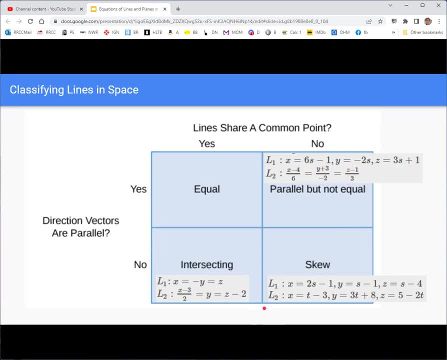 it is difficult to know how to tell them apart. Obviously they have different values for A, B and C, So that's how we know that the direction vectors are parallel, But telling whether they have a common point or not to see if they're intersecting. 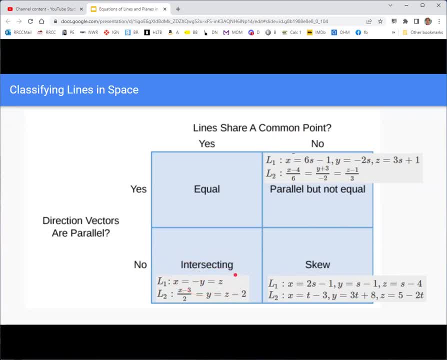 really involves solving them as a set of equations, And so we'll see it in another exercise how to do that. So if there is a T value or S value, a value for the parameter for which the two lines have the same coordinates, then they're going to intersect at that point. 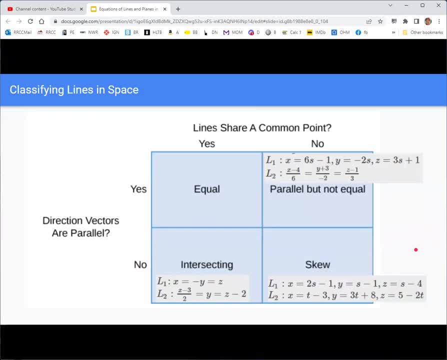 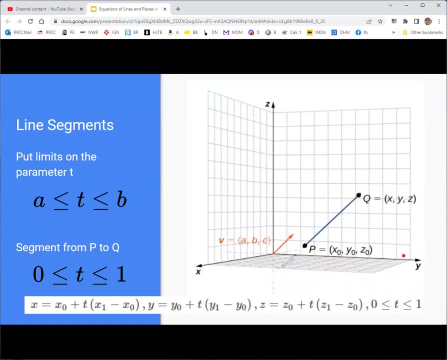 If there is no such solution, then they're skew, So it's not going to be immediately obvious just from looking at the equations. Now we can make an infinite line into a finite line segment by just limiting the parameter to a closed bounded interval. 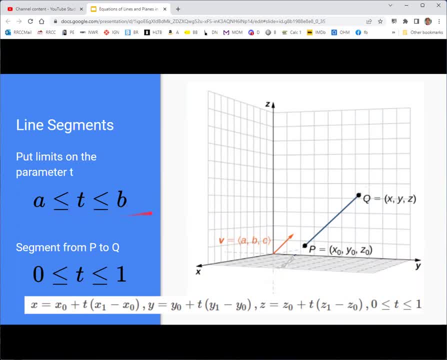 So, instead of going for T being all real numbers- T goes from A to B or, for instance, from 0 to 1, then that will give us a finite line segment And in particular, if T goes from 0 to 1, 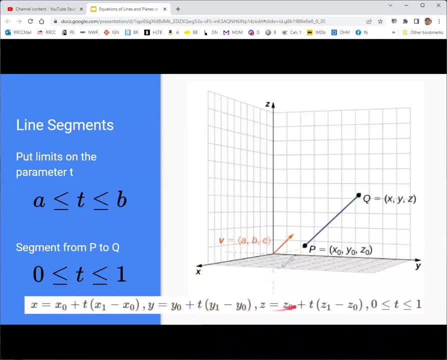 and you use the setup we had from before, where you start at X naught, Y naught, Z naught, and then you use the vector from P to Q, where Q is X1, Y1, Z1, then that will give you the line segment from P to Q. 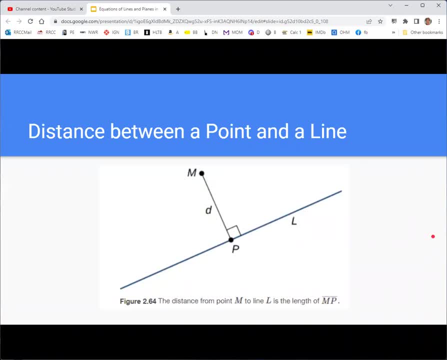 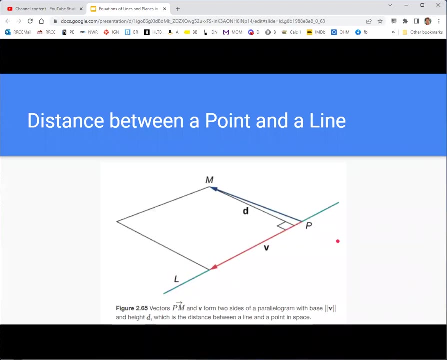 Right. So we've got the distance from a point to a line. So this, of course, is the straight line shortest distance. If we were to draw a straight line from the point to the line, it would be at a right angle to the line. 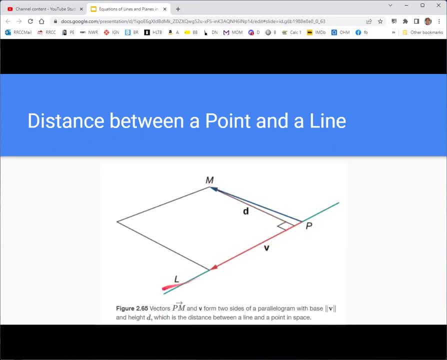 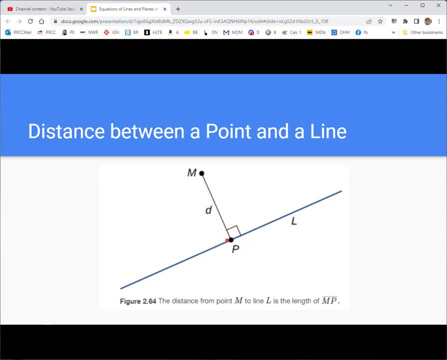 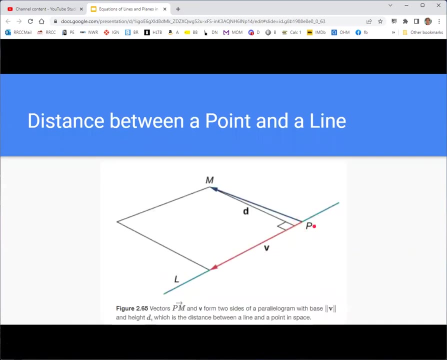 And in general we won't be able to find this point P, Then it would be obvious how to find D. So the way we find the distance D instead is we just grab any point on the line P, And so if you have the equation of a line, 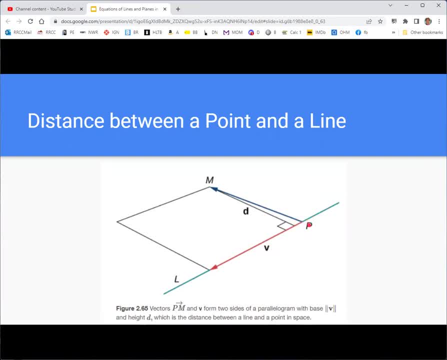 you can easily grab a point from its equations And we of course have a vector for the line, So we'll call that V And we basically create this parallelogram from the vector V that's on the line and then the vector that goes from the point P. 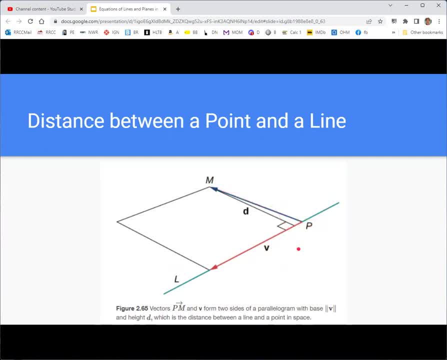 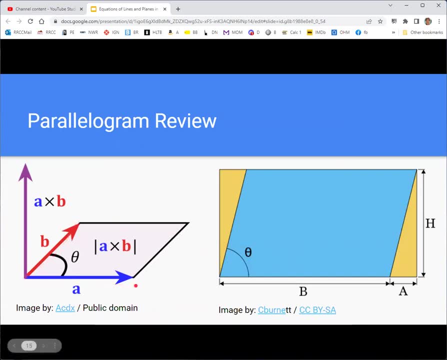 to the point M, that we're trying to find the distance between. Now you want to remember that the cross product of two vectors is equal to. Sorry, the magnitude of the cross product is equal to the area of a parallelogram. So in this picture here, 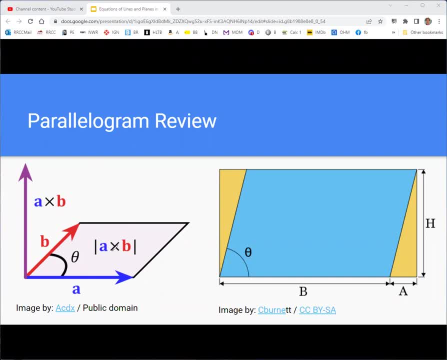 we're looking at the parallelogram formed by vectors A and B. The magnitude of A cross B is the area of that parallelogram. Now, we didn't mention this before, but the area of a parallelogram is equal to its base times its height. 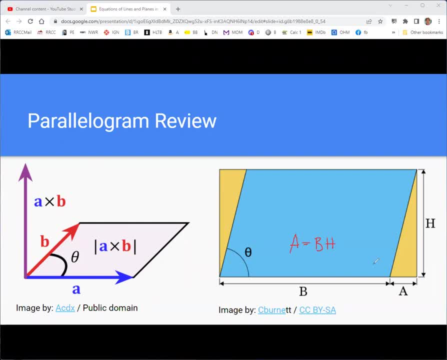 So B and H here, And this should make sense, because if If I sort of shifted this back like that and kept this fixed here, then I would just have a rectangle right And we know rectangle area is just length times width In this case. 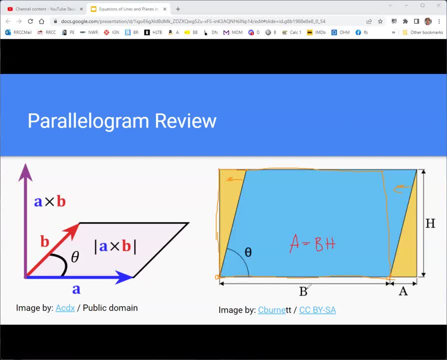 you could think of the length as the height and the width as B the base, And so all you've done is kind of skew or push the top of the rectangle to make it kind of slanted and make it a parallelogram, but its area is still the same. 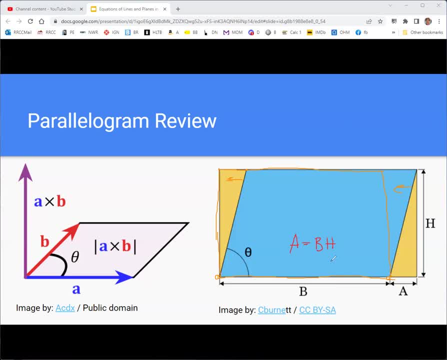 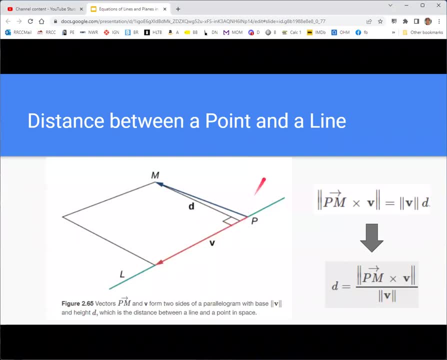 So area of a parallelogram is known to be the base times the height, And This is a parallelogram here, right, And So this is the parallelogram formed by the vector from P to M and the vector V. 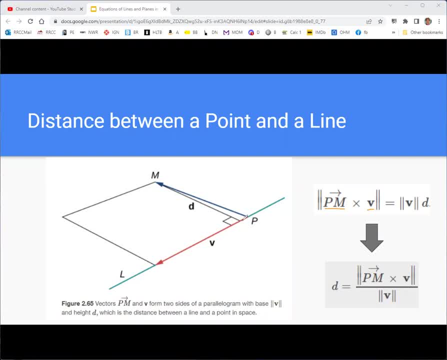 and that should be equal to the area of that parallelogram. And we know the area of the parallelogram is also equal to the base times the height. So in this case the base is the magnitude of V and the height is that distance. 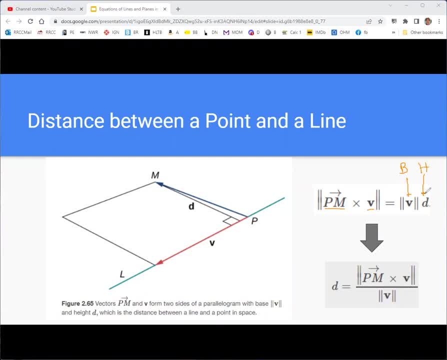 that we're trying to find So a lot of stuff here, but it basically is what we already know about the cross-product magnitude being equal to the area of the parallelogram, and then the well-known formula for the area of parallelogram. 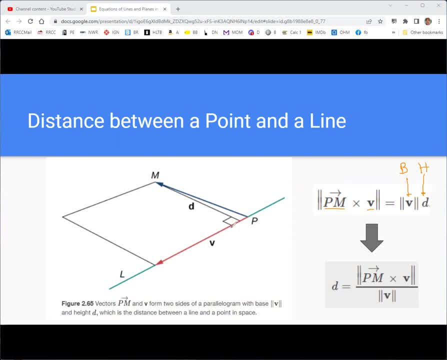 being its base times its height, and then just putting in V and D for those quantities, and then, of course, solving for D- which is what we wanted- by dividing by magnitude of V, And that'll bring you to this formula. 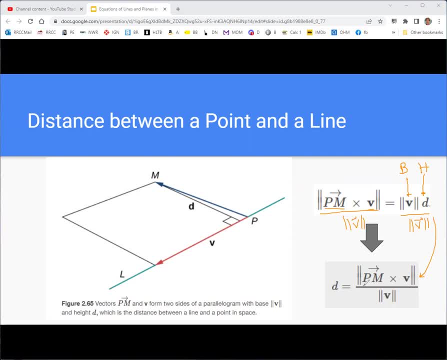 So this is the formula we used to find the distance from a point to a line. We need to create a vector from any point on the line to the point not on the line, And then we want to take the cross-product of that vector with the vector that's in the line. 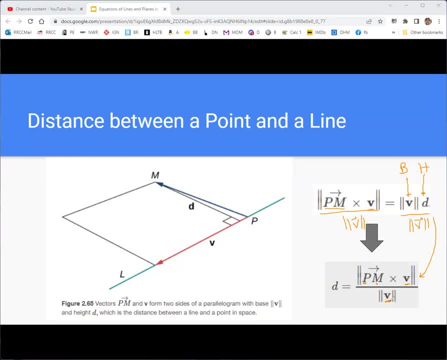 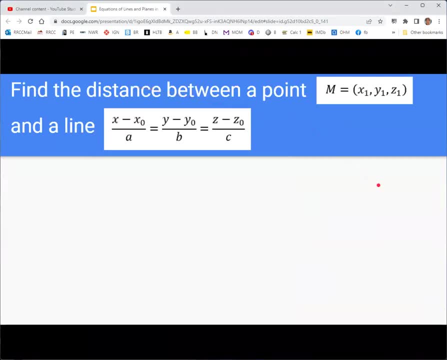 and then take the magnitude of that cross-product and then divide by the magnitude of the vector in the line, And then we want to take the cross-product of that vector to the point not on the line And then to say we had a point M. 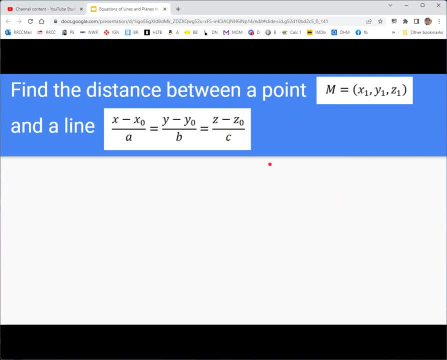 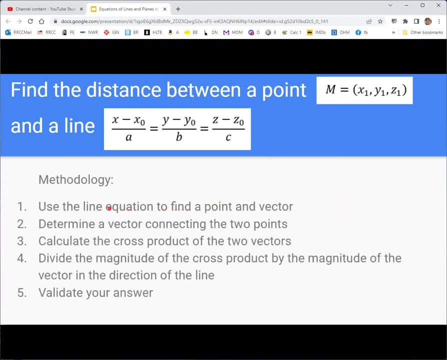 and a line given by this equation. I think we will do this in the methodology. So, using the line equation, no matter which setup you have, you should be able to find a point and a vector. Then you need a vector going from the point in the line. 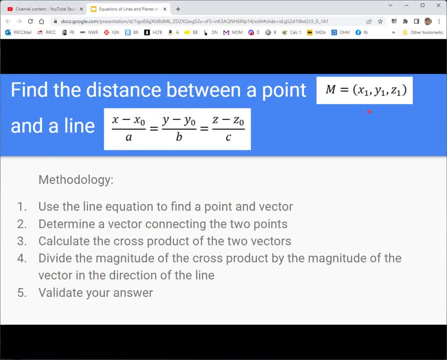 to the point off the line And then you get the cross-product of that vector we just created in step two with the vector that's in the line. And then we find the magnitude of that cross-product and divide by the magnitude of the vector in the line. 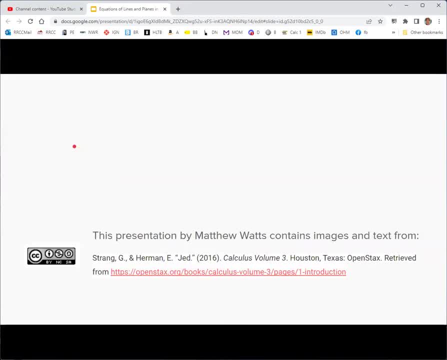 So we'll see that worked out in the methodology just next, And that's it for part one. This presentation by Matthew Watts contains images and text from Calculus Volume 3 by Jed Herman and G Strange. CC by NCSA OpenStack.